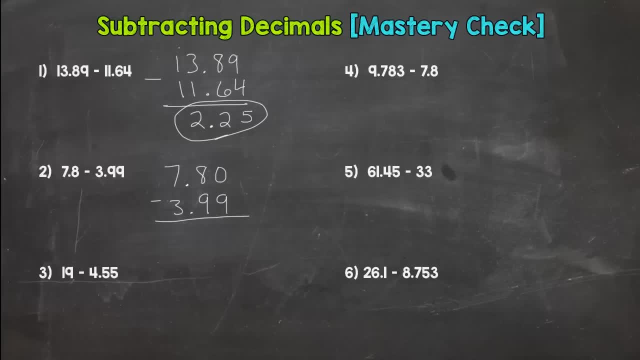 So we use a placeholder zero. Hopefully you didn't just drop that nine down. So we need to borrow here. Ten minus nine is one. Need to borrow again. Seventeen minus nine is eight. Decimal straight down: Six minus three is three. 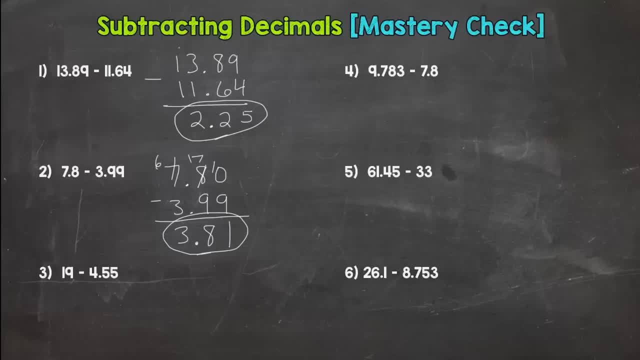 Three and eighty one hundredths Number three, We have a whole nineteen And hopefully we know that a decimal comes right after the whole number. This one will look really offset here, But that's all right. We put our placeholder zeros in. 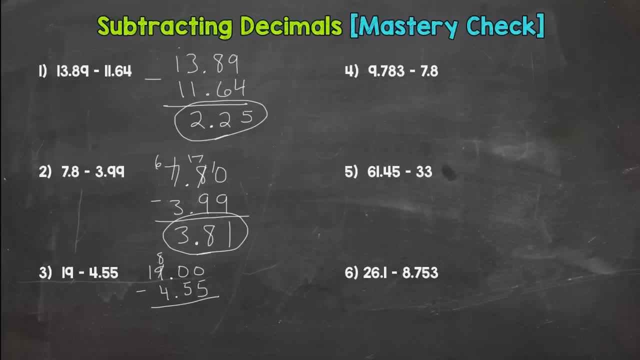 And we need a bunch of borrowing. This will turn to a ten, But we need to borrow from the ten. Ten minus five is five. Nine minus five is four. Decimal straight down: Eight minus four is four, And then one minus zero is one. 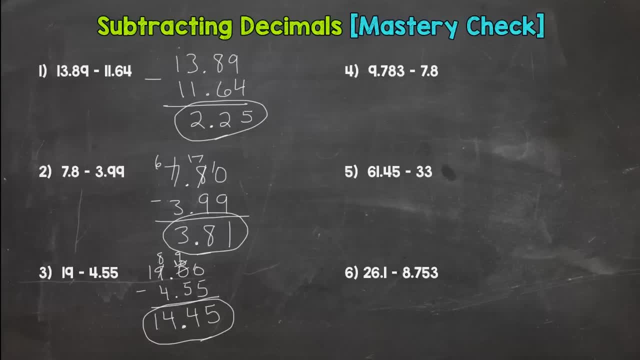 So fourteen And forty, five hundredths, And that is the halfway point. So hopefully three for three, All right. Number four: Let's line these bad boys up here, All right, Some placeholder zeros: Three minus zero is three. Eight minus zero is eight. 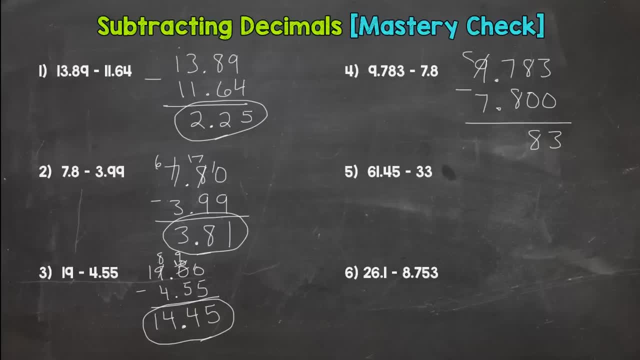 Cannot do seven minus eight. We don't want to go negative here, So we need to borrow: Eight minus eight is nine, Dot dot dot, Decimal straight down. And eight minus seven is one. So one and nine hundred eighty three thousandths. 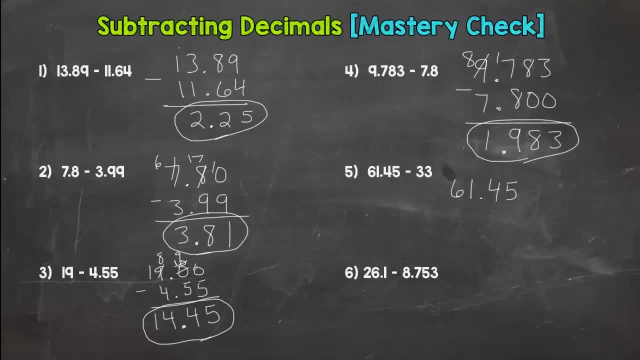 And on to number five. here Line up our decimals, Put placeholder zeros. Five, Four, Dot dot dot We need to borrow. Get to eleven minus three, which is eight. Five minus three is two, So twenty, eight and forty five hundredths. 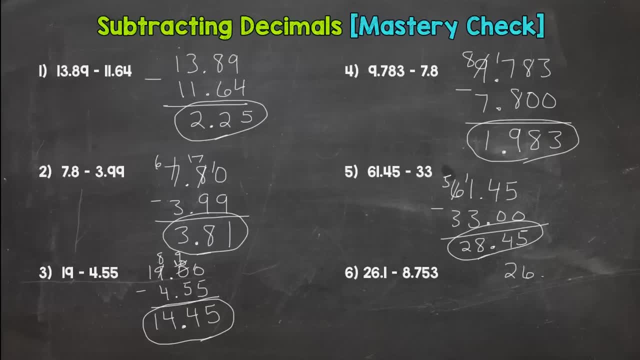 And then hopefully we finish strong here with number six. Line up our decimals Placeholder zeros. We need to borrow here. Take from the ten that's a nine. Ten minus three is seven. Nine minus five is four. We need to borrow again.